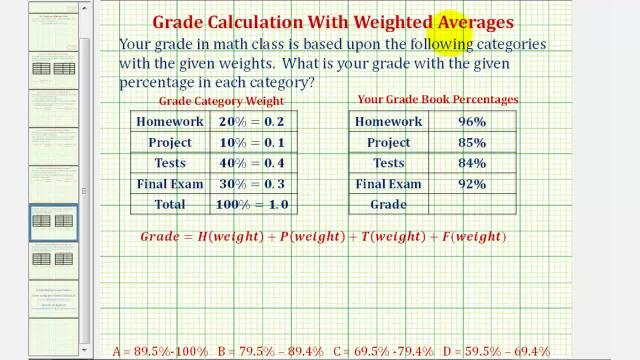 Welcome to an example of a grade calculation with weighted averages. Let's assume your grade in math class is based upon the following categories, with the given weights listed here on the left. So in your class homework is worth twenty percent of the grade, the project is worth ten percent of the grade. 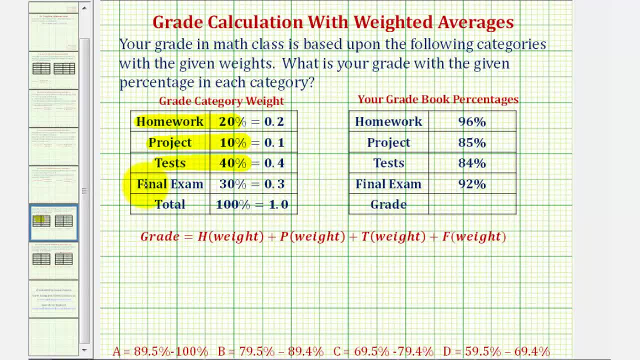 the tests are worth forty percent of the grade and the final exam is worth thirty percent of the grade. Notice how this total would be one hundred percent of your grade. We want to determine what is your grade with the given percentage in each category listed here on the left. So you've earned an average of ninety-six percent on the. 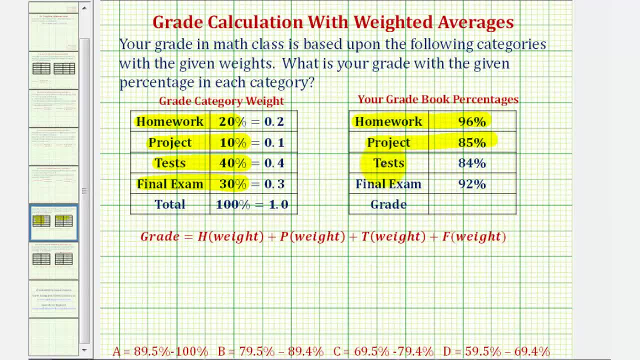 homework, eighty-five percent on the project, eighty-four percent on the tests and ninety-two percent on the final exam. So to perform a weighted average, we first want to convert all the percentages for each category into a decimal. Remember to convert a percentage to a decimal. 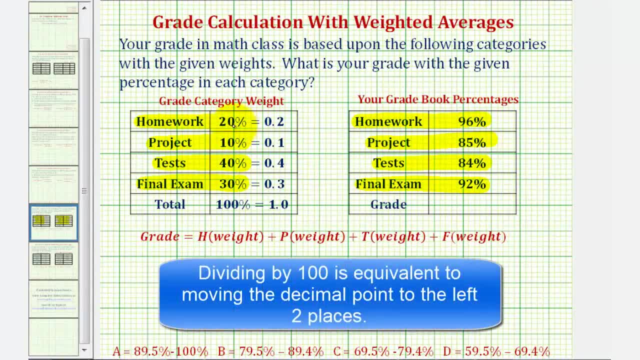 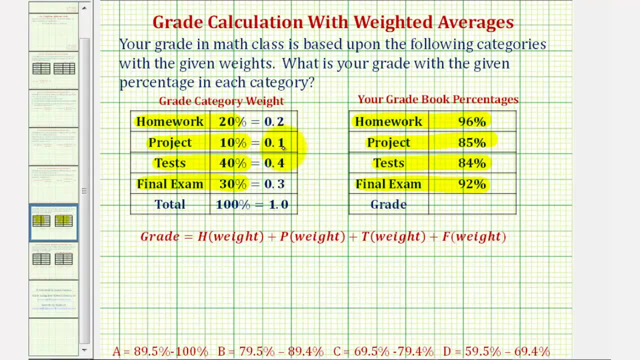 we drop the percent symbol and divide by one hundred. So twenty percent is equal to zero point two or two-tenths. ten percent is equal to zero point one or one-tenth. forty percent is equal to zero point four or four-tenths. 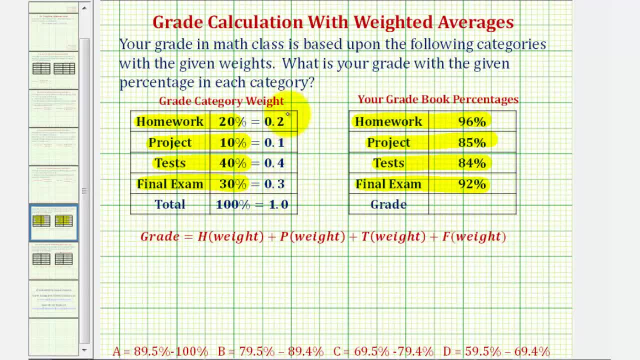 and thirty percent is equal to zero point three or three-tenths. So what this is telling us is, looking at the homework average of ninety-six percent, this is worth two-tenths of the semester grade. The project grade of eighty-five percent is worth one-tenth of the semester grade. 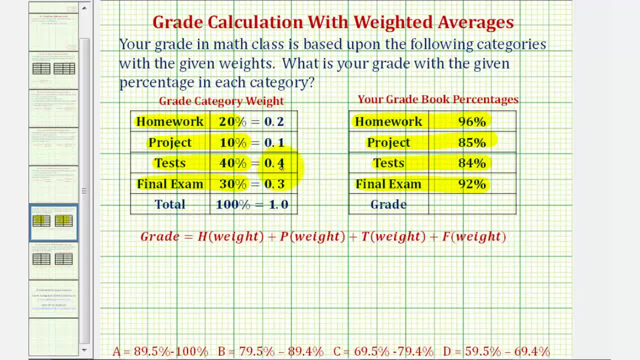 the test average of eighty-four percent is worth four-tenths of the semester grade, and so on. So to find the grade for the course using these weighted averages, the grade will be equal to the homework percentage, which is ninety-six percent. 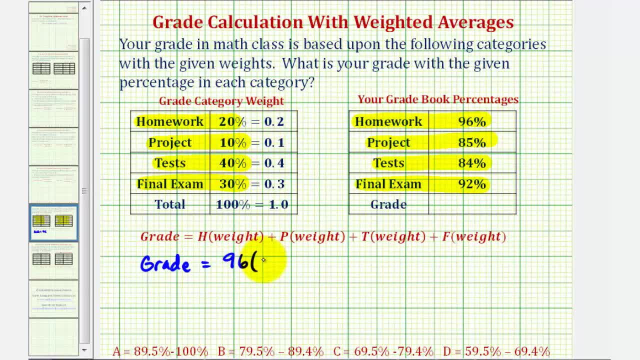 We'll leave off the percent for the calculation times the weight of zero point two, plus the percent for the project, which is eighty-five percent times the weight of one-tenth or zero point one, plus the test average of eighty-four percent. 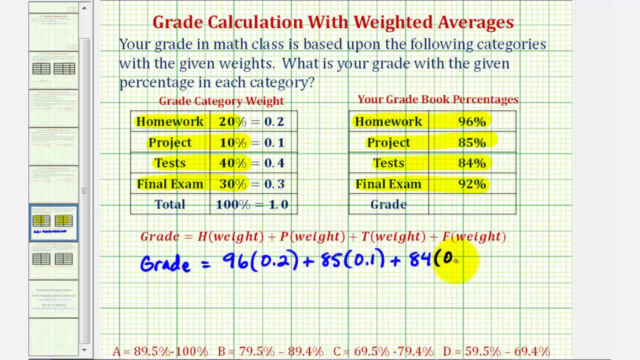 times the weight of zero point four or four-tenths, plus the final exam grade of ninety-two percent times the weight of thirty percent or zero point three. So the sum of these products will give us the grade for the course.